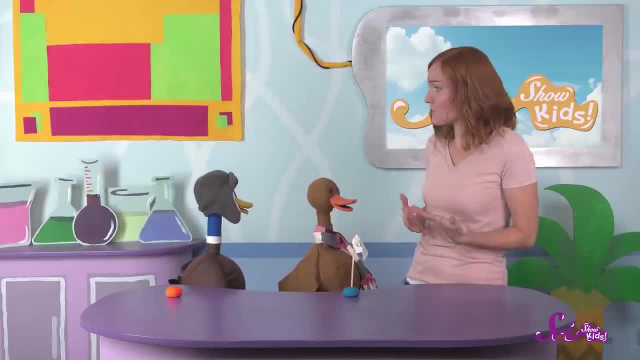 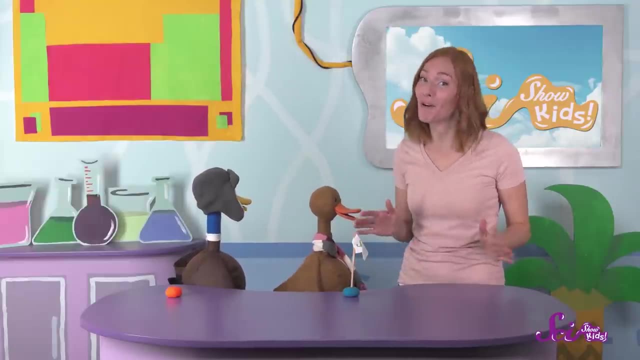 Jumping is like that too, So can you think of a way you could give yourselves a speed boost when you jump? We could make our muscles stronger, That's true, And practicing jumping is a great way to get super strong, But that takes time, and there's something else that you could do that would help you get faster right now. 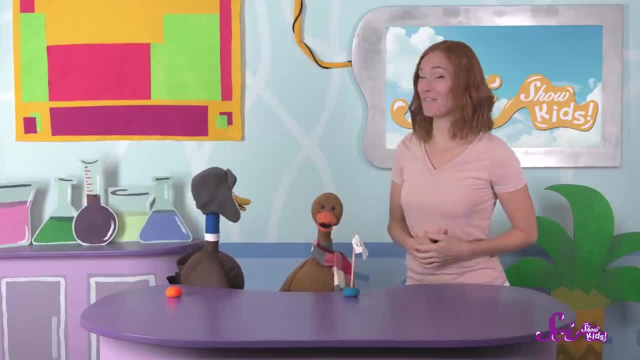 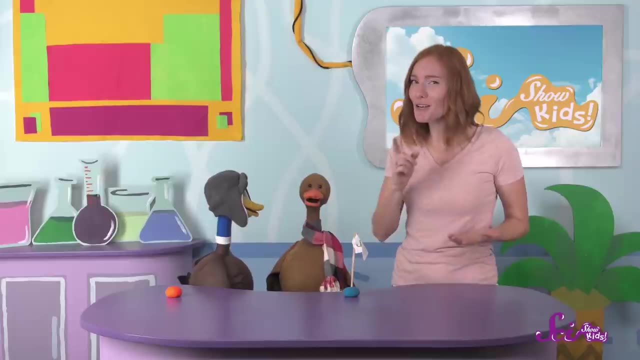 Oh, I know We could do a run-up first. Great idea, Webb, Webb. if you're already moving really fast, when you jump you'll go farther than if you just tried to jump from standstill. So that's one tip that you can try, and I can think of one more. 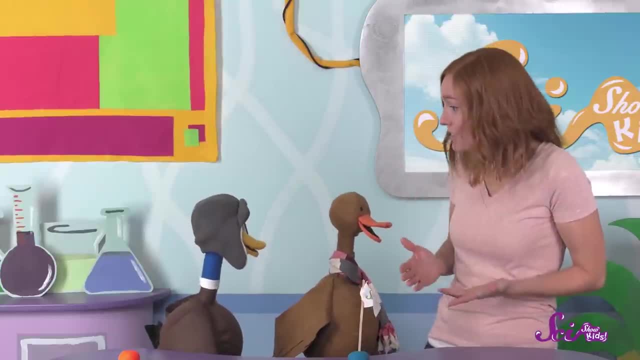 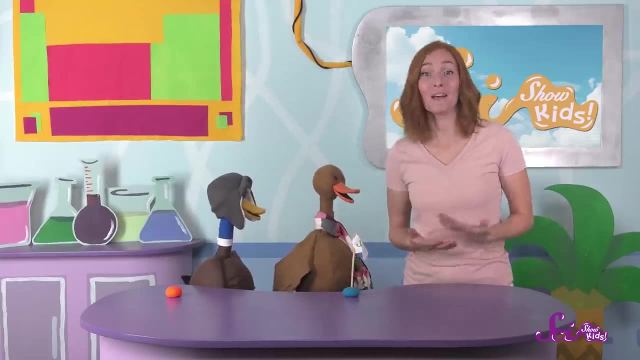 I noticed you're both jumping straight ahead of you instead of up. Well, of course we are, Jessi. We're trying to jump forward as far as we can, not as high as we can. That's true, Bill. If you want to go far, jumping forward is important. 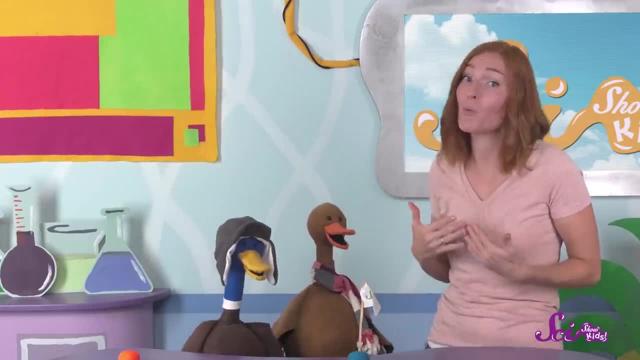 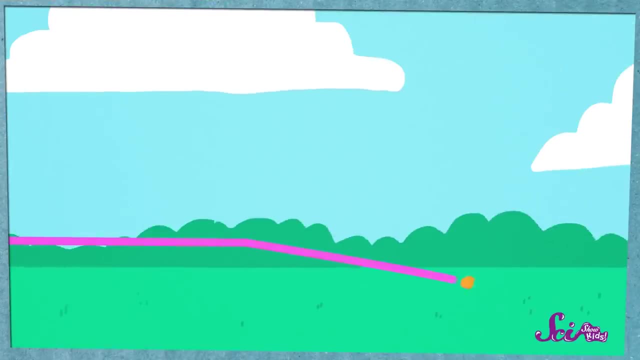 But it's also important to jump up a little too. so you're on more of a diagonal. Think about that softball again. What happens if you throw it straight ahead of you? It might go kind of far, but pretty soon it will hit the ground. 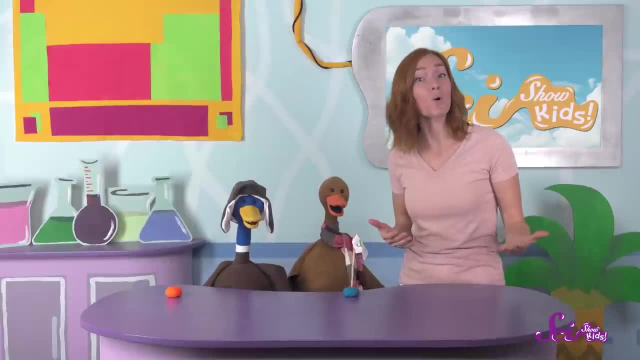 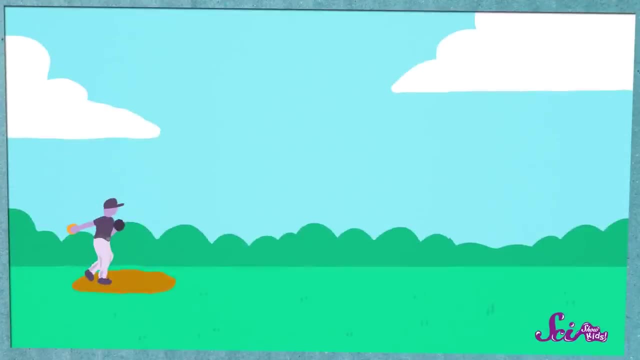 It will hit the ground and roll instead of moving farther through the air. It keeps rolling because it had lots of speed left, but it was so close to the ground that it landed really quickly If you throw the ball forward and up on a diagonal. 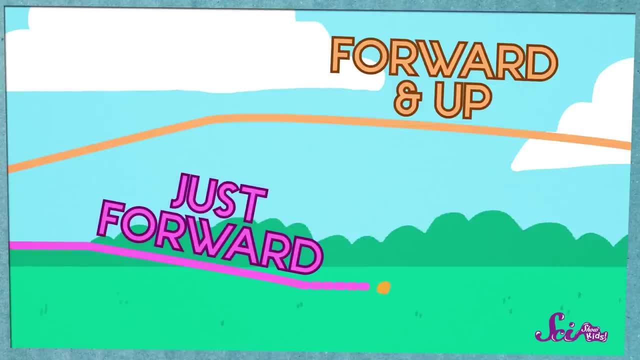 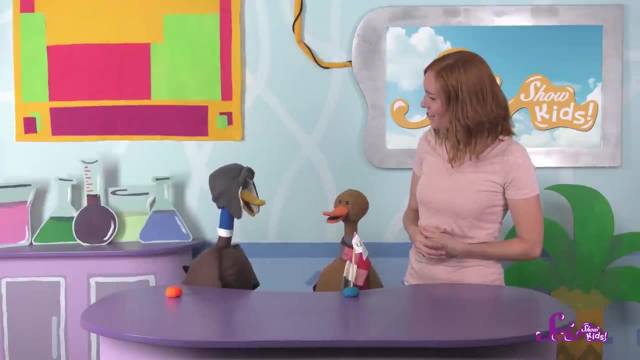 it will take much longer to fall to the ground and in the meantime it has a chance to move much farther through the air. So if you jump on a diagonal, you'll also go farther. Okay. so to jump farther than that flag, all I have to do is run up, then jump on a diagonal. 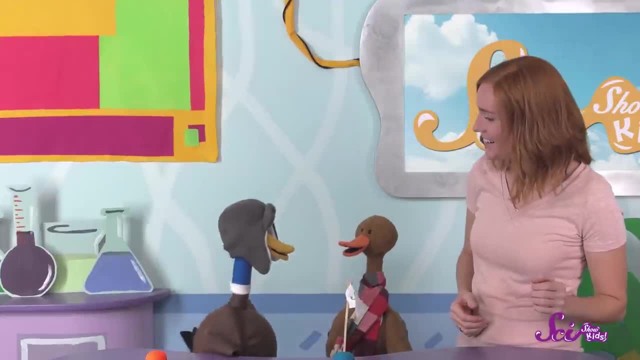 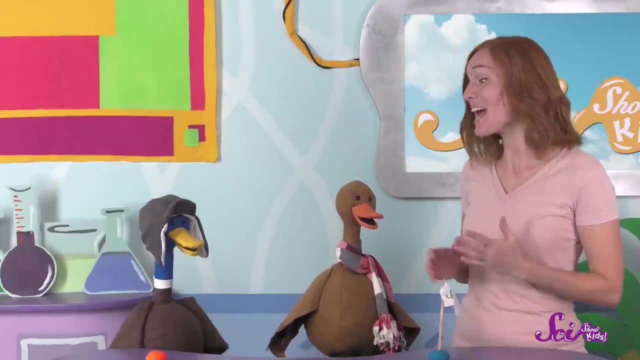 I bet it'll help. I'm gonna try it. I did it. Yay, That's fantastic. Webb, Can I use these tips too, Of course, And I also think that you'll be able to jump farther than you could before. 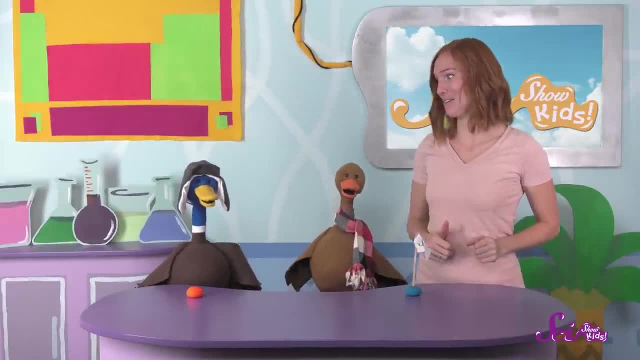 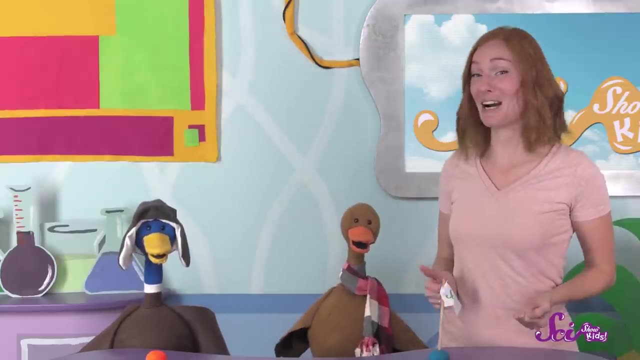 Why don't you both keep taking turns and see how far you can go? Yeah, Thanks for the help. Jessie, You bet This is a great game. You get to run and jump and play all at the same time. When you play, you get your blood pumping and your muscles moving. 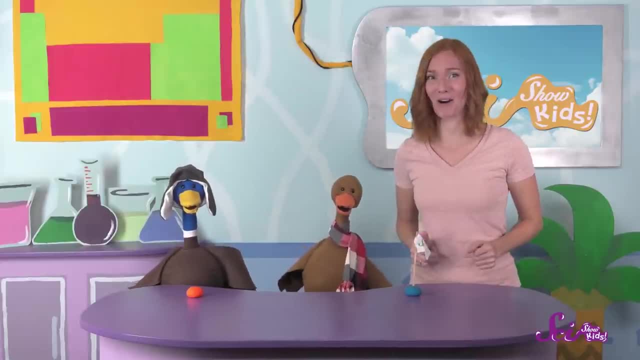 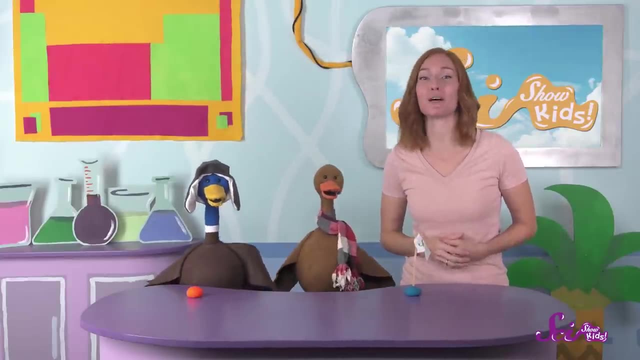 Your heart beats faster, you breathe harder and you get stronger. That's all really important, And so is getting your yearly checkup at the doctor. With over 600 muscles in your body, it's important to make sure they're all working the way.